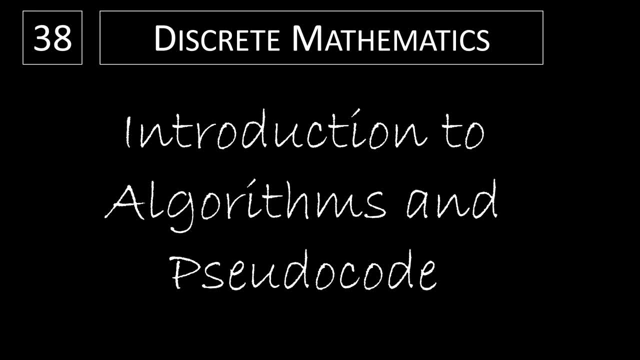 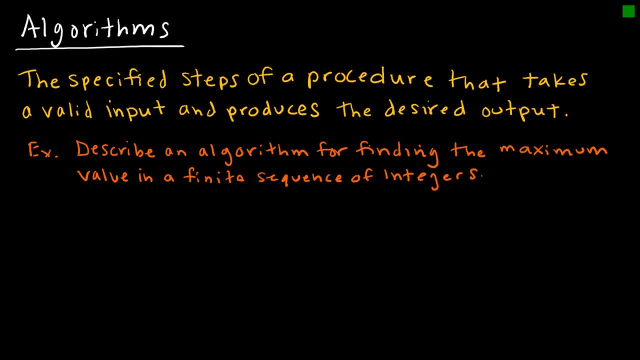 This video is an introduction to algorithms and pseudocode. So an algorithm is just a specified steps of a procedure that takes a valid input and produces the desired output. For example, how might we describe an algorithm for finding the maximum value in a finite sequence of integers? So obviously? 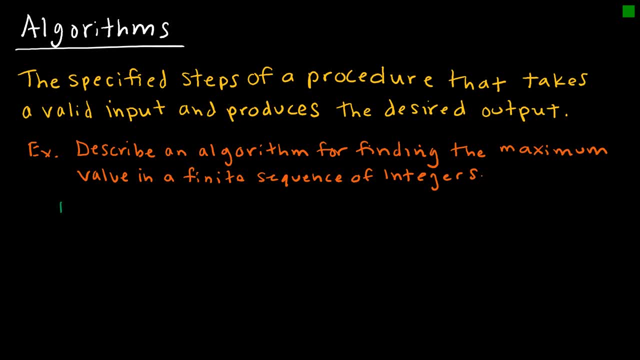 there's no one right answer for this, but essentially what we want to do is we want to start by setting the first value equal to our temporary- our- sorry that said out, our temporary- maximum. so essentially we're saying the first value in the sequence is our temporary max. then what's going to? 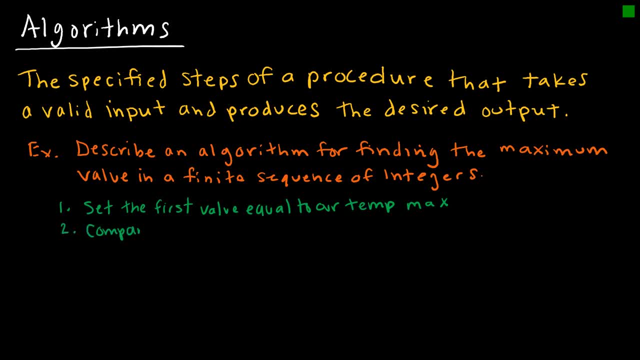 happen? we're going to compare the second integer to our temporary max. if the integer is greater than our temporary max, what are we going to do? we're going to set it as our new temporary max. so what's going to happen if it's not greater? otherwise, ignore. essentially, we're just going to repeat these steps until no. 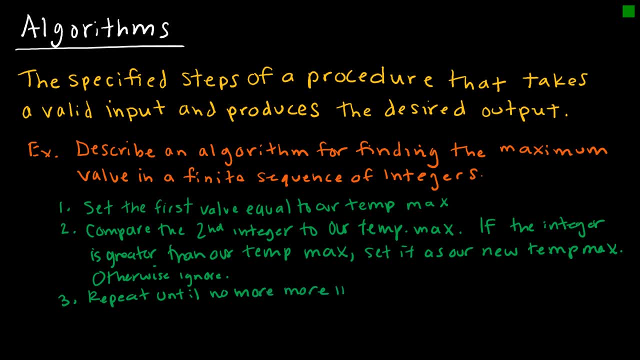 more integers exist. now you might be thinking: well, this seems very involved and I'm not quite done yet, I've got one more step. but you might be thinking: well, this seems stupid, I'm just going to look at the last one and I'm going to go ahead and do that. 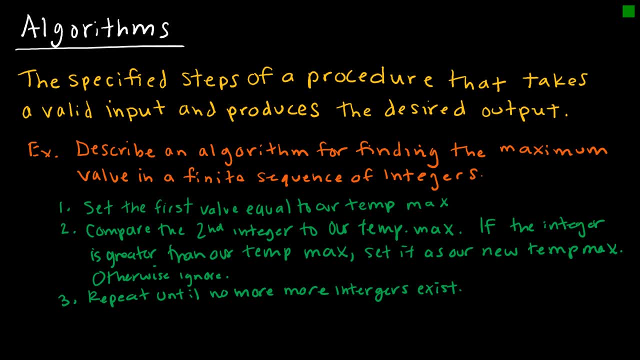 remember, an algorithm gives us specific, specific steps to follow, and it really has a lot to do with computer programming. computers aren't just going to look at a list and say this one's the biggest. computers look at algorithms which can handle much larger groups of data than we can. so our last is: 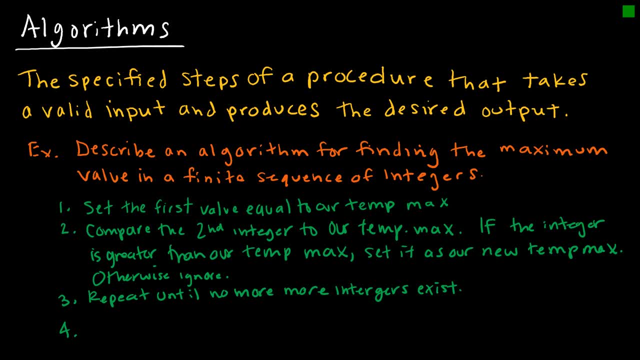 basically just telling us how do we know what the maximum is? so When the process is over, when the algorithm terminates, and it terminates again when we run out of numbers, the temporary max is the maximum integer. So this is an example of an algorithm that finds the maximum value in a finite sequence of integers. 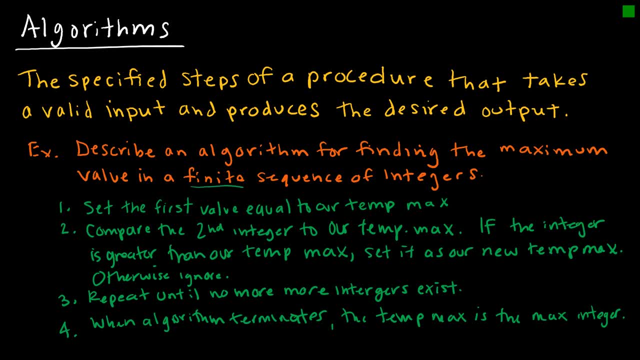 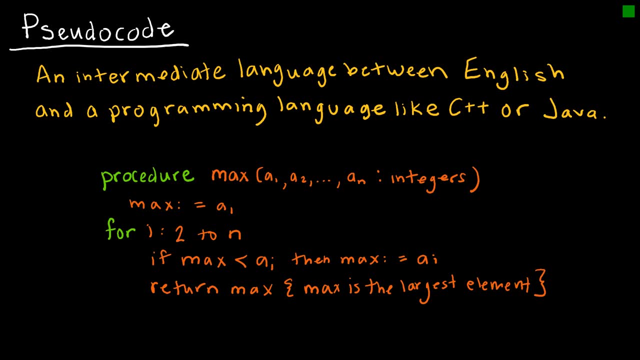 Obviously there is no value if it's an infinite sequence of integers. So we're going to look a lot at the pseudocode in this lesson and the next several lessons in Chapter 3, Section 1 of your textbook, And pseudocode is just sort of an intermediary step. 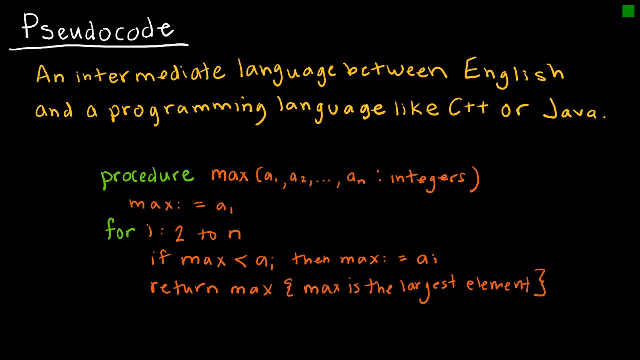 So we're not going to look at Java programming or C++ or any of those, But this is sort of a step in the direction That you would go if you were going to actually code your program to come up with the maximum integer. So notice, here I've called this the procedure. 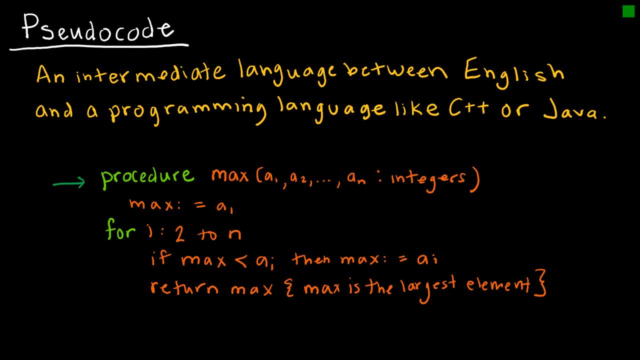 And the procedure is going to give me that I'm finding the max. It's telling me what values I'm going to use, which are the values in a sequence, And that they are integers, And that I'm looking for, That I'm setting the maximum equal to that first value. 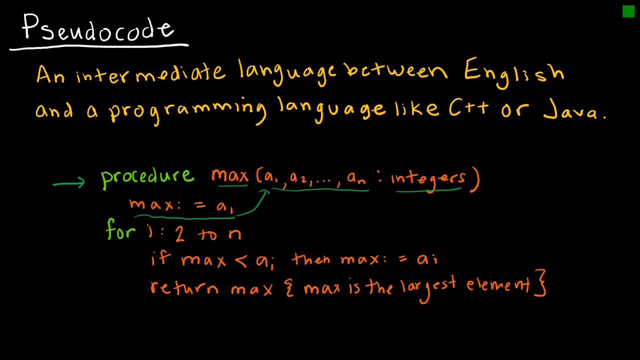 So that's sort of step one in the steps that I previously showed. Then it says hey for all of the other integers, so 2 through n. So for all of these values, if the max is less than a i, which means if the max is less than our new value. 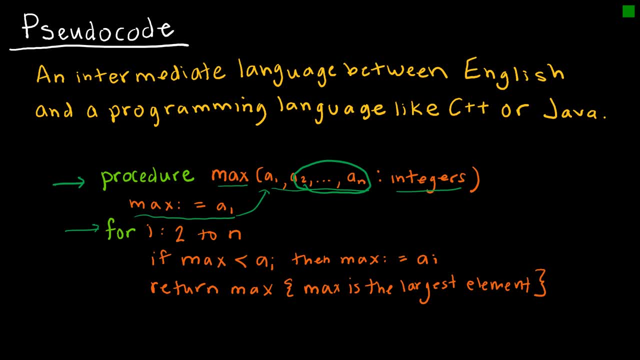 Because our new value is a sub 2,, a sub 3,, a sub 4,, etc. Then our new max is that value Return. this is what tells us what the final output would be. So the return is the max, where max is the largest element. 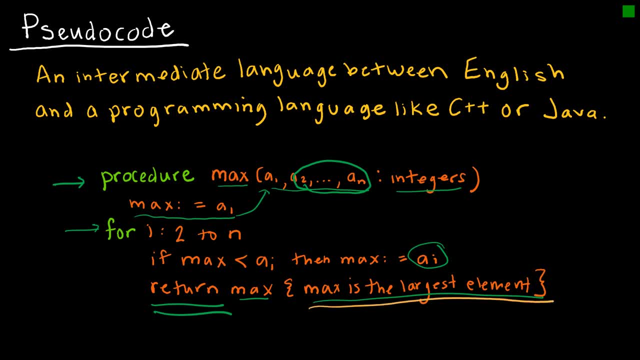 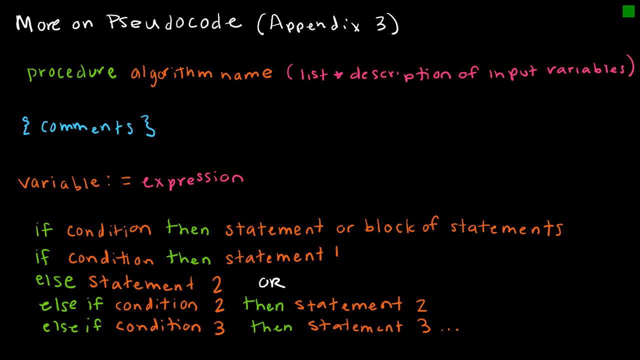 Now I want to point out that this here is just a note. It's a comment that helps us as a person understand, But it's not something that the computer would read. There is a whole lot on pseudocode in your textbook, in Appendix 3.. 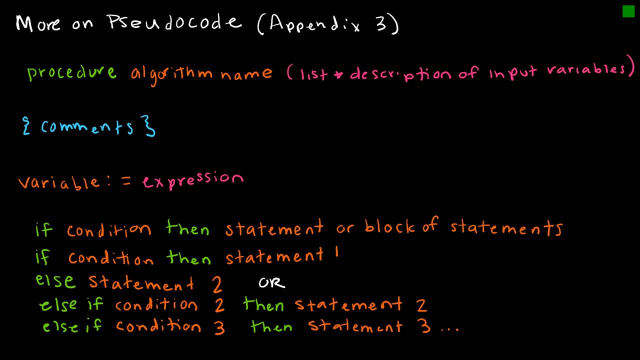 And I've just- I've just- listed some of them here just so that we're used to or somewhat familiar with things that we might see in the pseudocodes. for the rest of the algorithms we'll talk about in this section. So notice, if you're going to do a procedure, the procedure, we would first write procedure and then we would say what the algorithm name is. 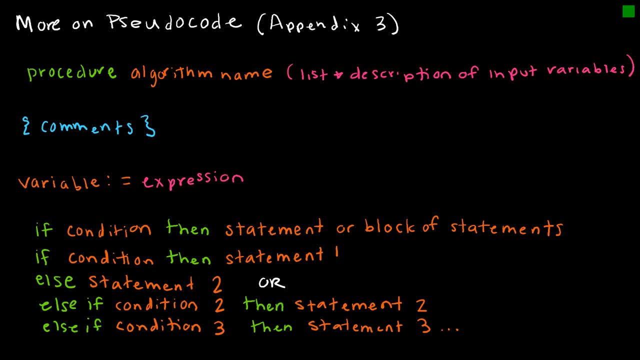 So on the last one I said max, And then this is the list and description of the input variables. And that is what I did before I said: hey, we're using a 1.. A 2,, A 3,, etc. 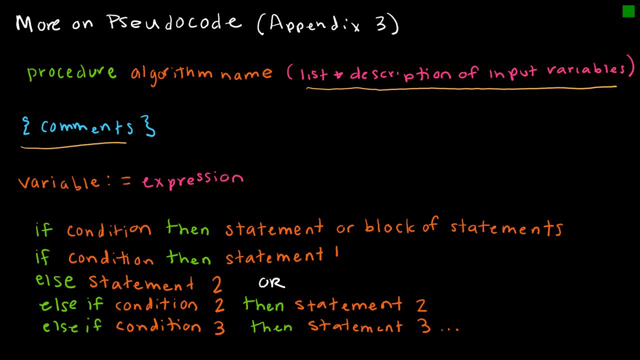 And those are all integers. Here is a comment. That's what happened at the end when I had that in brackets. Again, comments are not read by computers, They're just for people. If we're using a variable, we use variable, then a colon and then equals and then the expression. 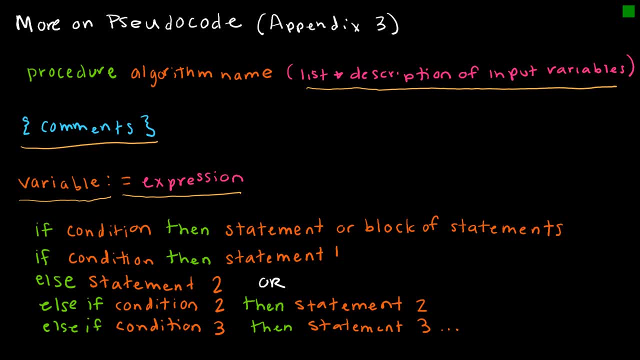 And then you've got a lot of conditional statements And we should be familiar with conditionals. But it might just be an if condition Then statement, or if condition, then block of statements, or it could be if condition then statement 1,, else statement 2, or if condition, then statement 1,, else if condition 2, then statement 2,, if condition 3, then statement 3,, etc. 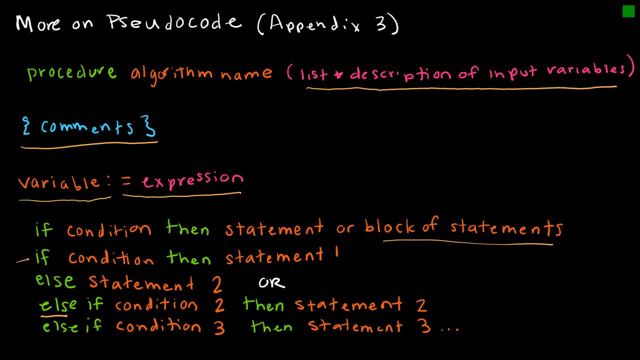 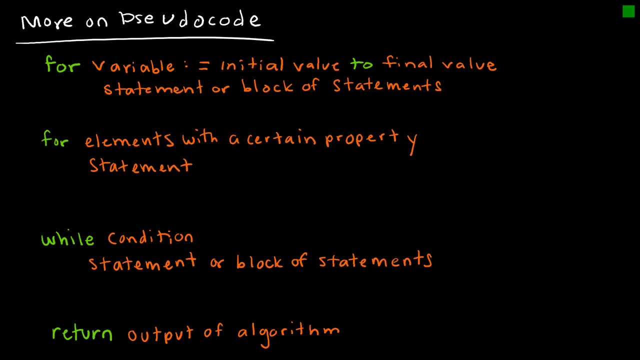 So the else just says: hey, if statement, if it's not this one, then it's going to be this one, or then it's going to be this one. A few more Commands in pseudocode you might see. So this one is for some variable. 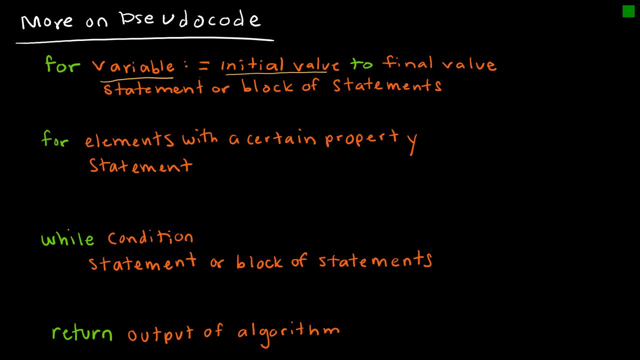 So for some variable equal to an initial value, to some final value. And so remember, before we said for I and we said that started at 2 to N, So that told me that that subscript was 2 through N. And then it tells us what's happening: statement or block of statements.